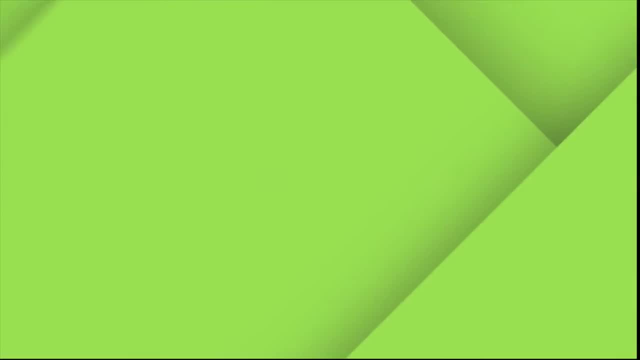 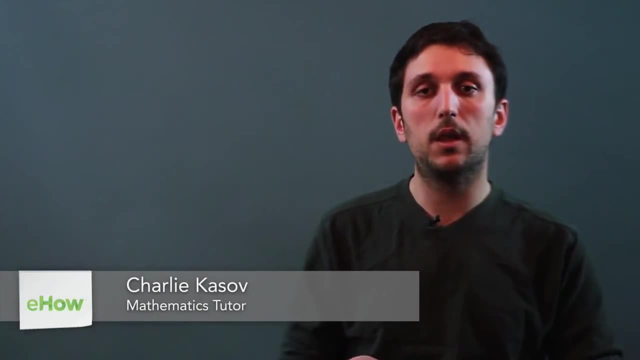 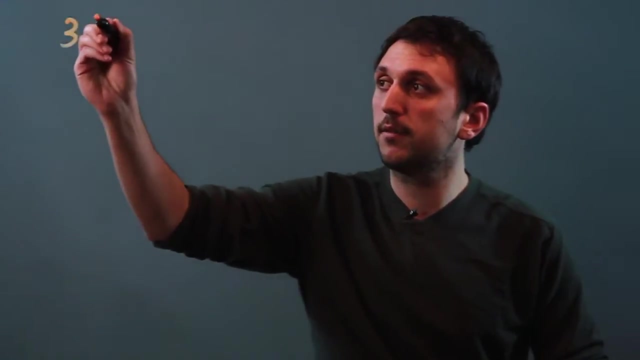 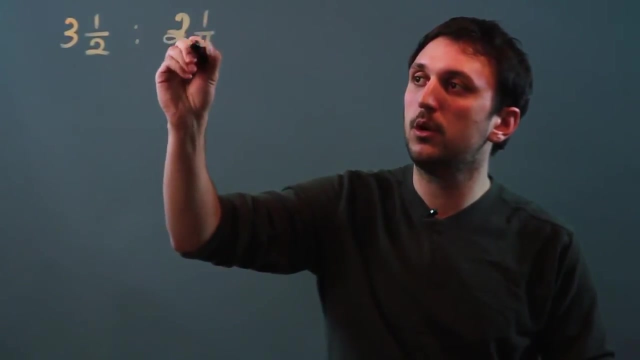 Hi, I'm Charlie Kasov. I'm a math teacher And today we're going to learn how to do ratios with mixed numbers. Now, the goal with mixed numbers is to turn them into proper fractions. Let's take two mixed numbers: We have 3 1⁄2 and we have 2 1⁄4. So let's say we want to have these as a ratio: 3 1⁄2 to 2 1⁄4.. 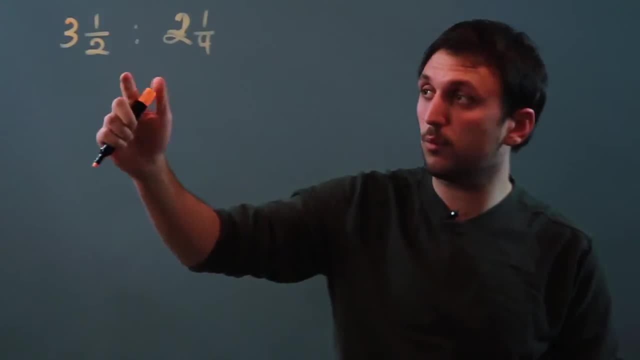 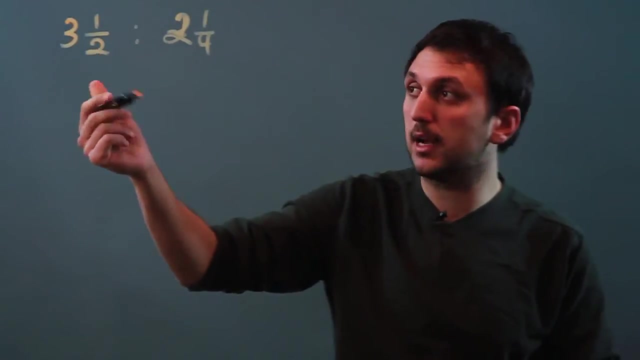 Well, we're going to need to change these into proper fractions. Right now, what you have is a whole number and a proper fraction, so they're mixed. To change this one to a proper fraction, we say, okay, well, we want everything over 2.. 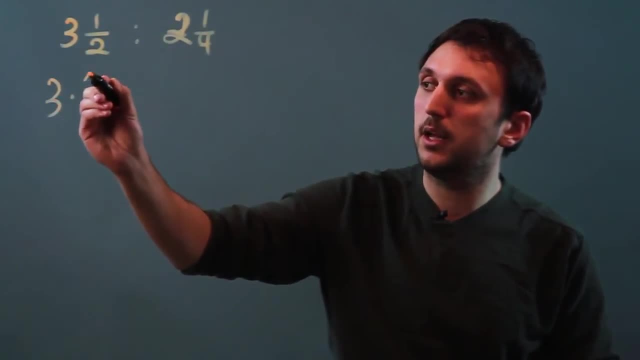 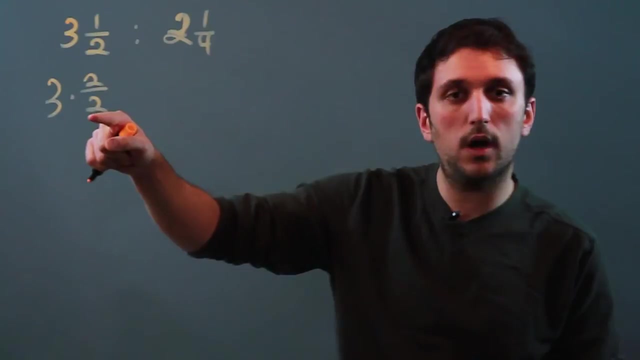 So we'll take 3 and we'll multiply it by 2 over 2, which is really just 1.. So this is called rationalizing. We change it to the number we want without changing the value. So 3 times 2 over 2 is 6 over 2.. 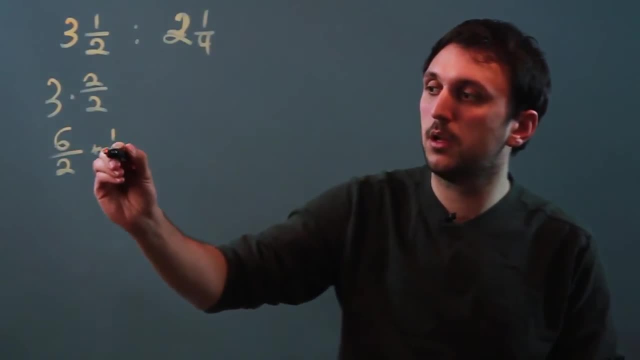 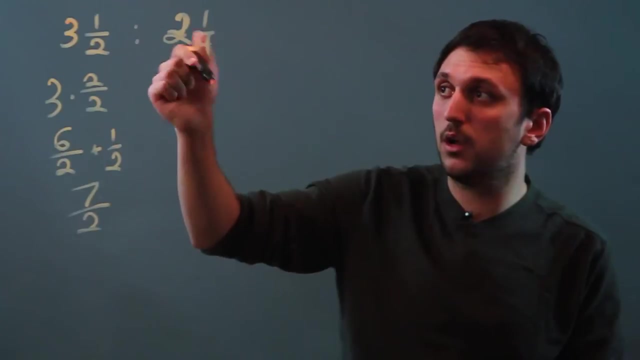 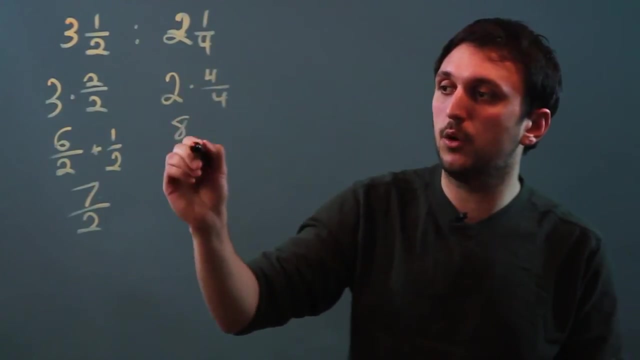 Plus, that extra 1⁄2 up here is going to give us 7 over 2.. Then over here we have a denominator of 4, so we have this 2. We're going to multiply it by 4 over 4, which gives us 8 over 4.. 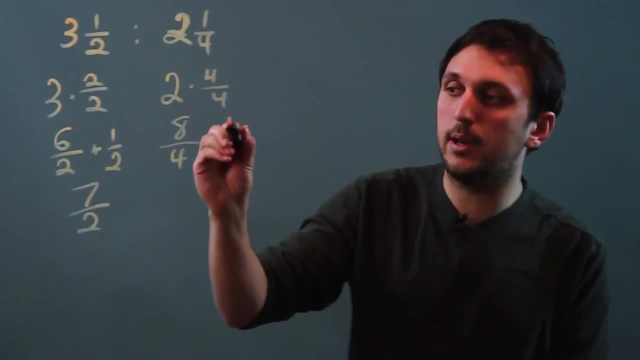 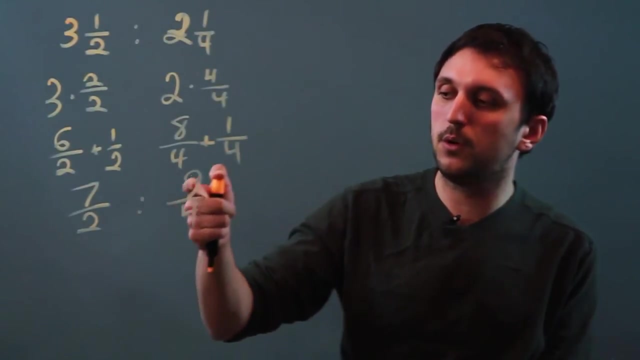 And we still have this extra 1⁄4 hanging out. so we add 1⁄4, and we get 9 over 4.. So now we have a ratio of 7 over 2 to 9 over 4.. 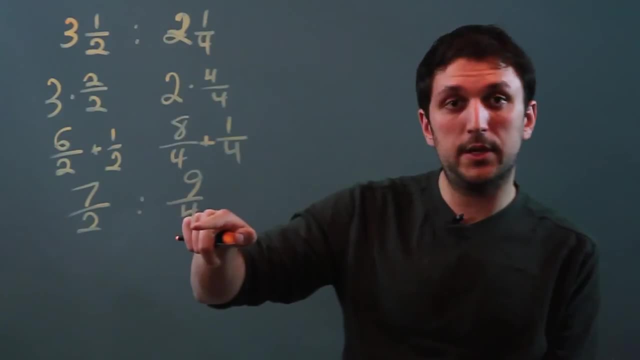 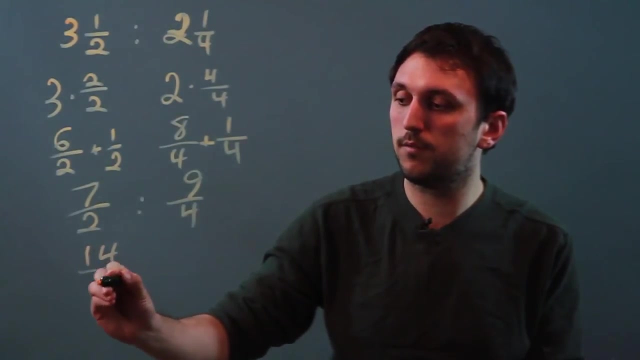 Can we do anything more? Well, we have a denominator of 4 and a denominator of 2.. Maybe we double this and we say 14 over 4, which is the same thing as 7 over 2, is to 9 over 4.. 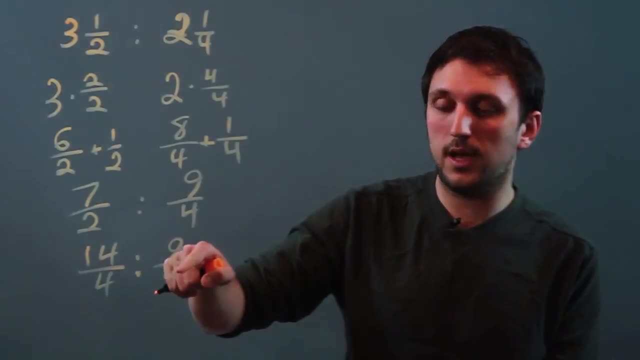 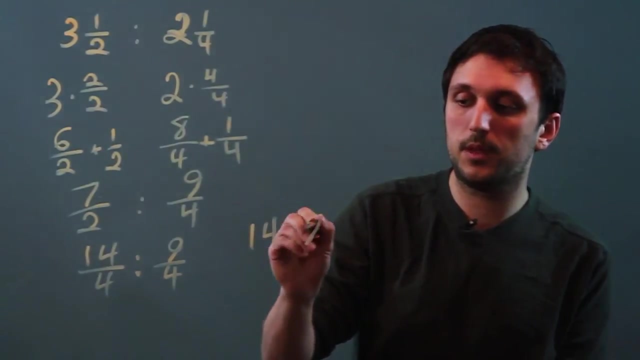 Now this ratio looks a lot cleaner: 14 over 4 to 9 over 4,- which we can then simplify because the bases are the same to saying 14 to 9.. So I'm Charlie Kasov And you just learned how to do ratios with data. You just learned how to do ratios with mixed fractions. Thanks a lot.